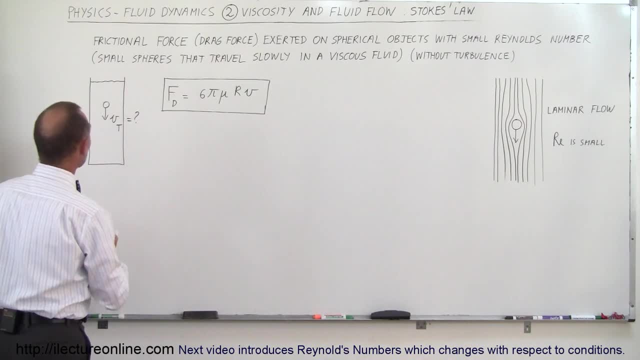 zero. Now, what are all the forces on the object? So let me use a different color. Well, for one thing, there will be a buoyancy force acting upward, So there'll be a buoyancy force in the upward direction. There'll be the force of gravity, mg, acting downward, And then there's 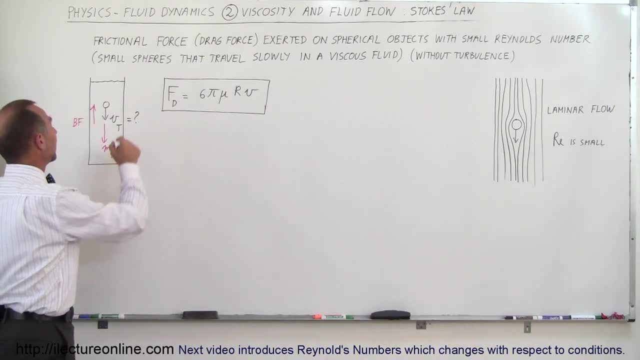 that third force that we haven't talked about before. in a situation like this, It'll be the drag force, which is, of course, moving the opposite direction, or I shouldn't say moving, but it's acting in the opposite direction to the motion of the marble or the sphere, And so it would be f? sub. 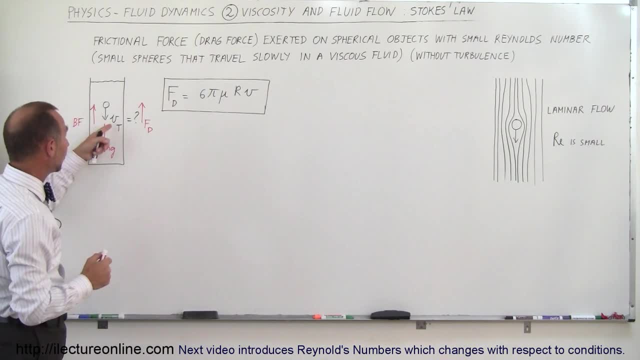 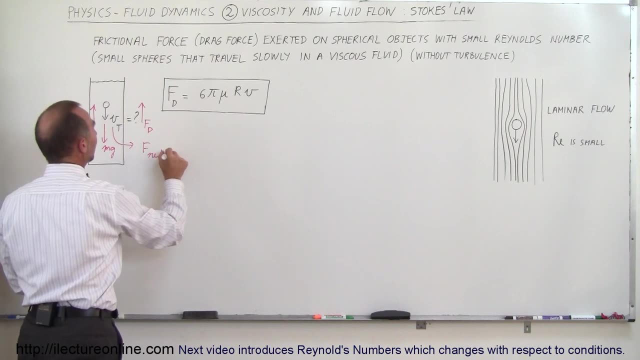 d, And we then realize that when terminal velocity is reached, the net force will be equal to zero. So, at terminal velocity, f sub d. So what we can say then is that the buoyancy force plus the drag force is equal to the. 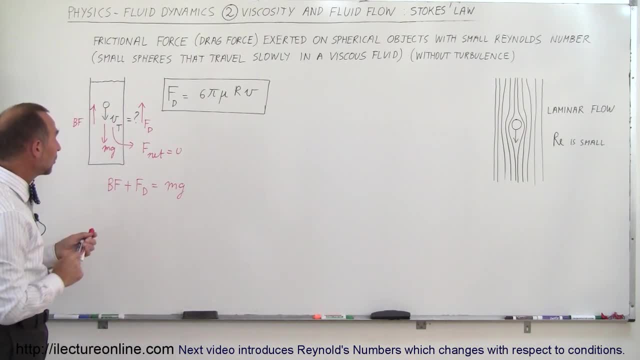 weight of the marble. All right. So what we're going to do now is we're going to move the buoyancy force to the other side. We're going to write that the drag force is equal to the weight of the marble minus the buoyancy force, And now we're going to put down what those things are equal to. 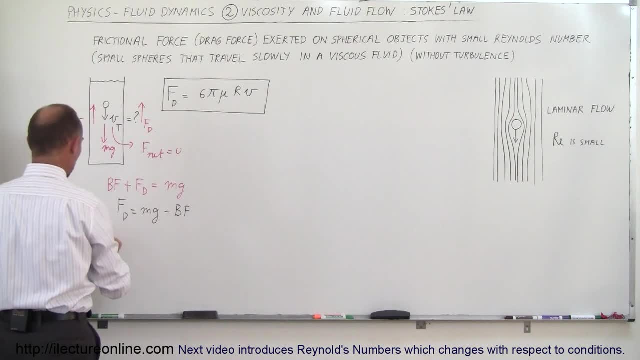 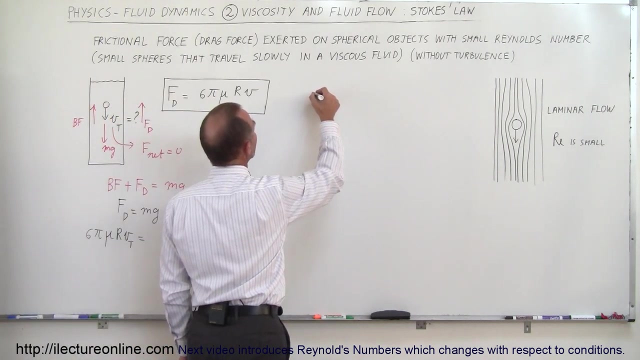 Well, first of all, because of Stokes' law, we now know what the drag force is. We know that the mass is equal to six pi mu times, the radius times, the terminal velocity, The weight, mg. but we want to convert the weight into something we can relate to. Let's see here. We know that the density of an 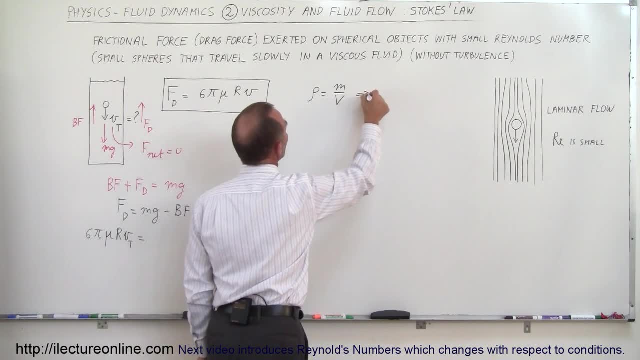 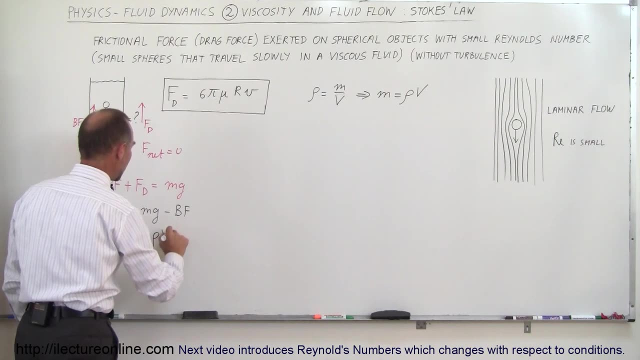 object is equal to the ratio of the mass divided by the volume, which means that the mass can be written as the density times the volume. So in this case, instead of mass we can write rho vg of the object. This is of the marble. 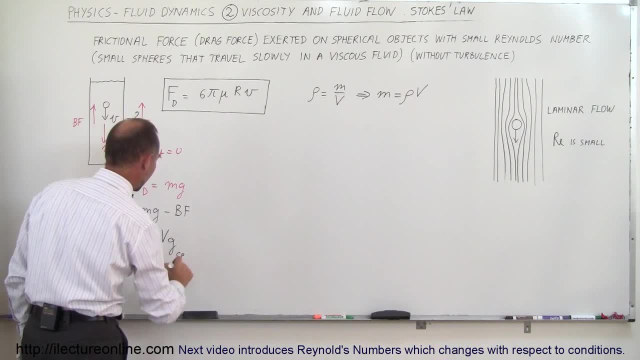 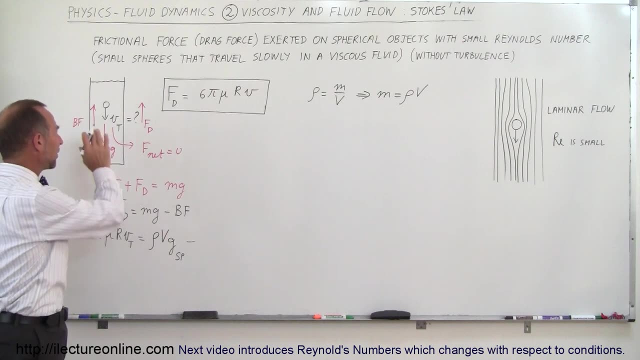 Yeah, let's see here We'll call it sphere sp for sphere minus the buoyancy force, And of course the buoyancy force is equal to the weight of the displaced liquid. In that case that will be the rho vg of the liquid. All right, So the volume is the same for both, G is the same for both. 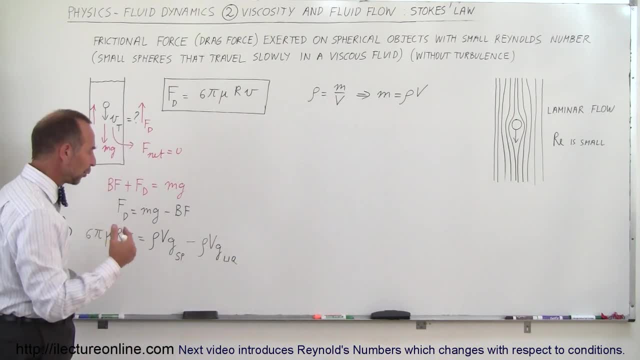 of course It's the constant of gravity. Remember, the volume of the sphere is four-thirds pi r cubed. So let's go ahead and factor out a vg, And that means we have six pi times mu times r times the velocity. terminal velocity is equal to. 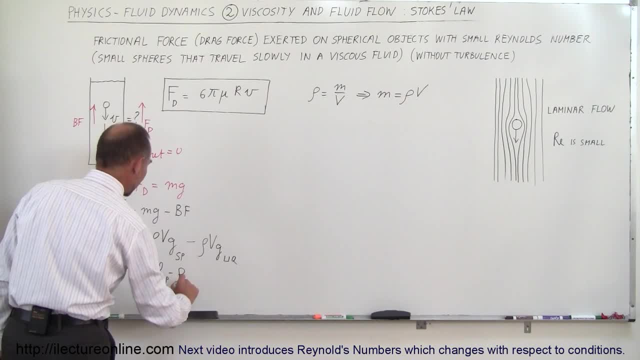 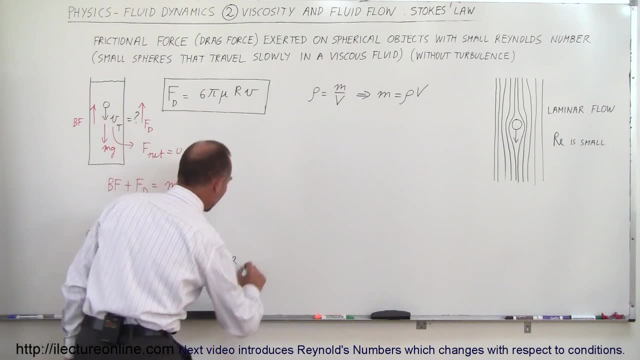 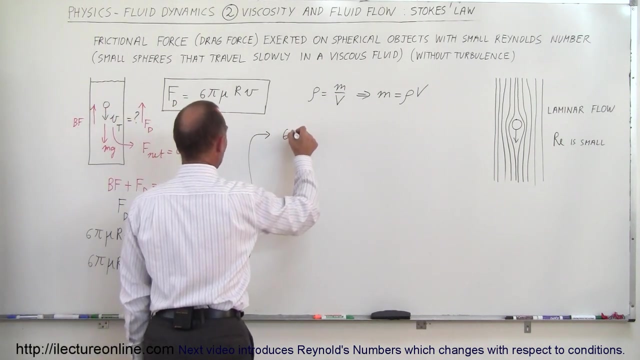 the density of the sphere minus the density of the liquid, multiplied times the volume times g. And of course, since I'm out of room, let me come up here, And then we can write this again And we'll replace v with what v is equal to. So we can write that six pi mu. 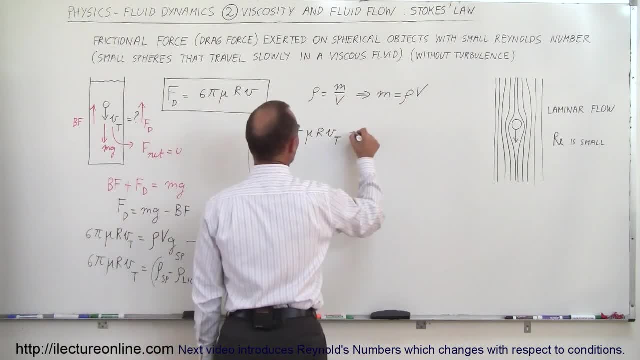 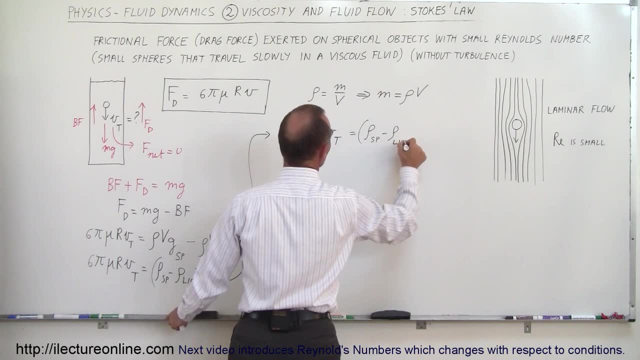 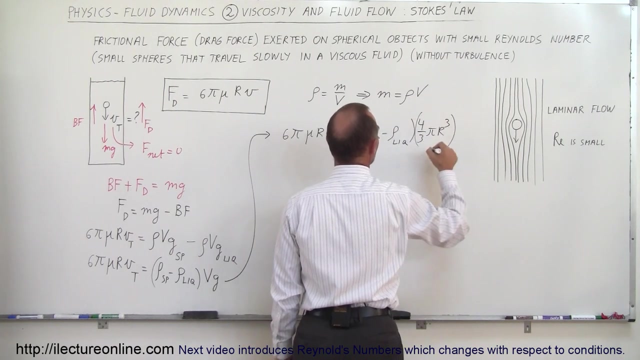 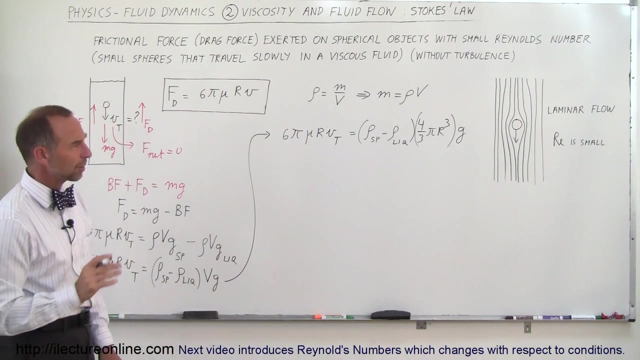 times r times the velocity is equal to the difference in the density of the sphere minus the density of the liquid times, the volume, which is four-thirds pi r cubed times the acceleration due to gravity. All right, Now we should be able to solve that equation for terminal velocity. We. 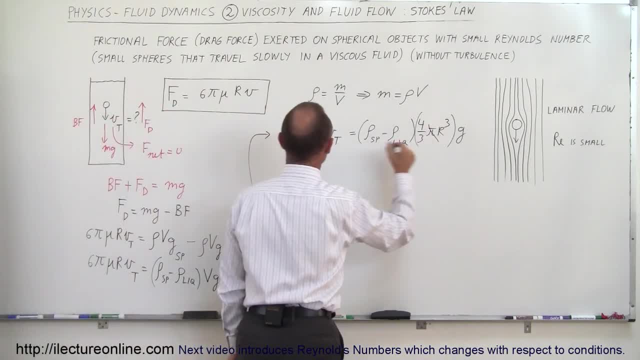 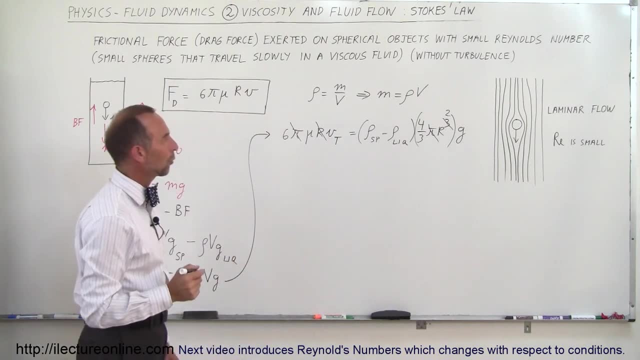 could probably simplify a few things. Notice that we have a pi on the left side, we have a pi on the out. We have the radius of the sphere here and we have three of them there, so that changes from r cubed to r squared. We still have a 6 here. We can bring the 6 to the other side and write 4 over. 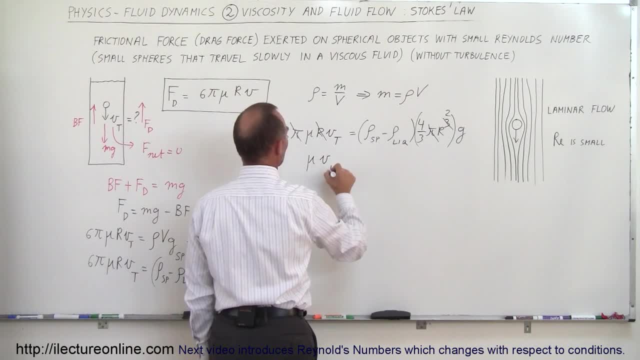 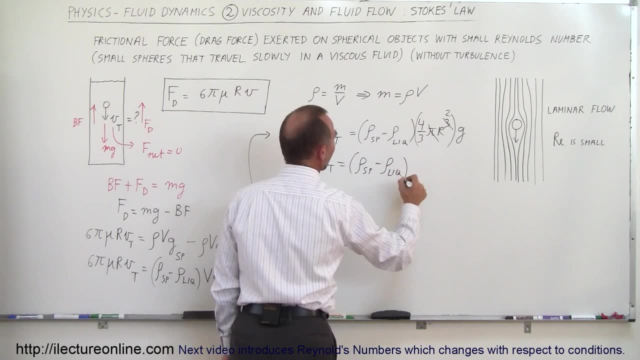 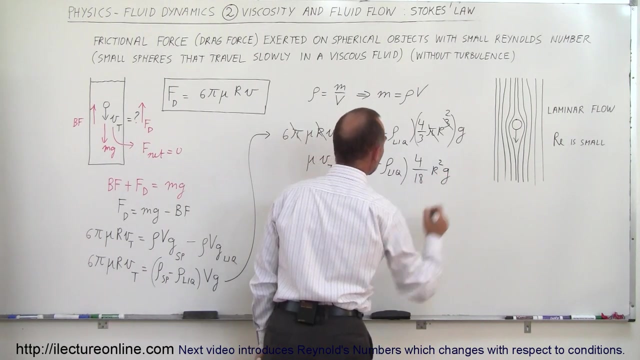 18.. So now we have mu. terminal velocity is equal to the difference in the densities sphere minus the density of the liquid, times 4 over 3 times 6, which is 18, times r squared g. Now we can take: 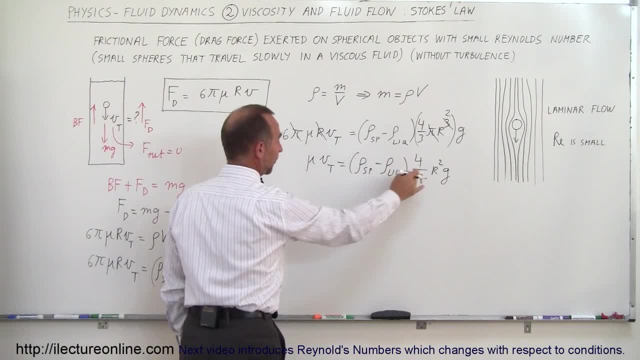 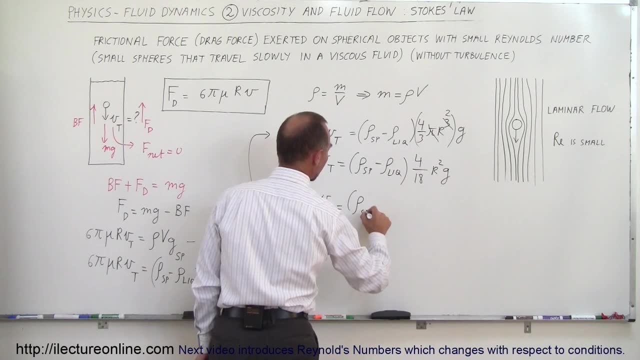 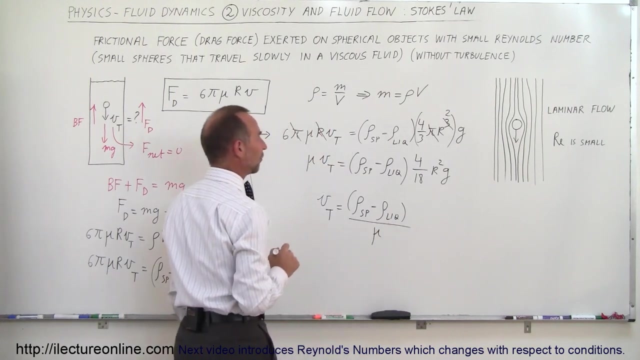 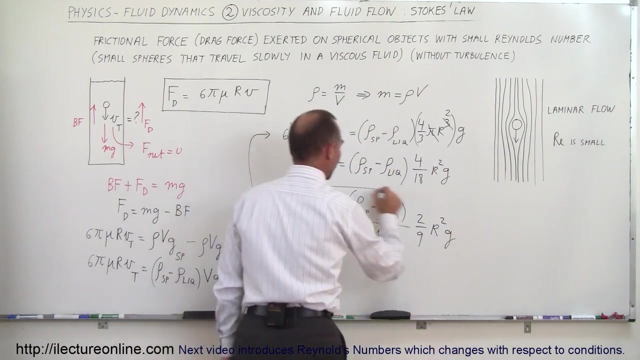 the coefficient of viscosity. bring it down there, simplify that and now we have an equation for the terminal. velocity v sub t is equal to the difference in the densities divided by the coefficient of viscosity times 2 over 9, times the radius squared, times g, And this is now the equation of the terminal. 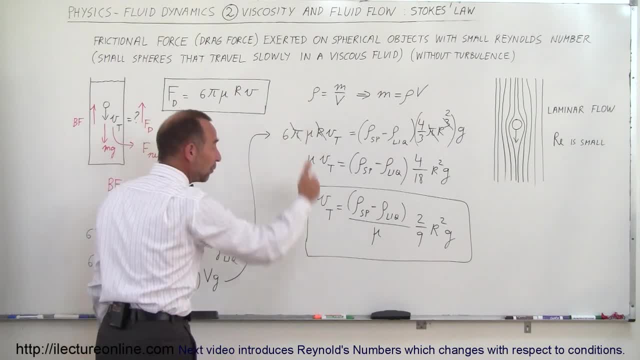 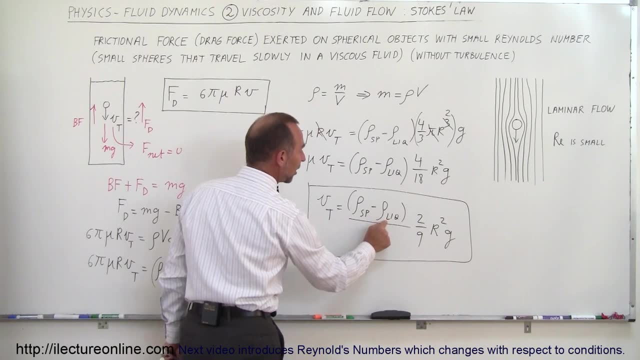 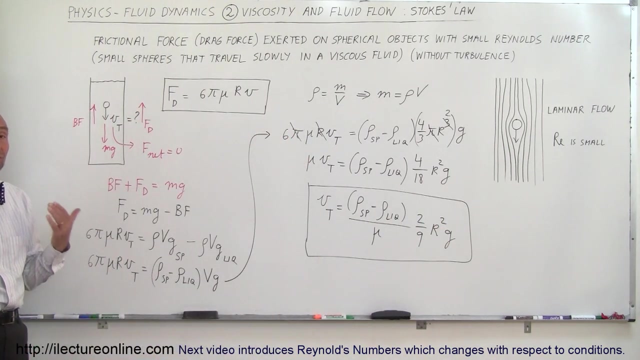 velocity of a spherical object moving through a viscous liquid, where r is the radius of the object. this is the density of the object, this is the density of the liquid, the viscosity of the liquid and the acceleration due to gravity. And so Stokes' law now gives us two things. It gives us